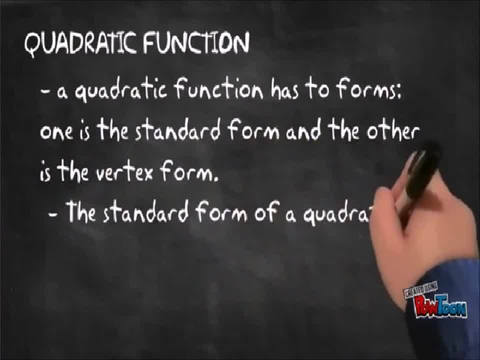 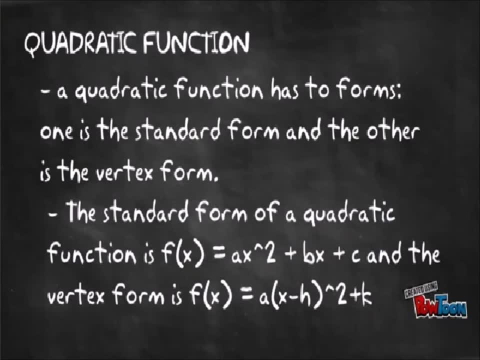 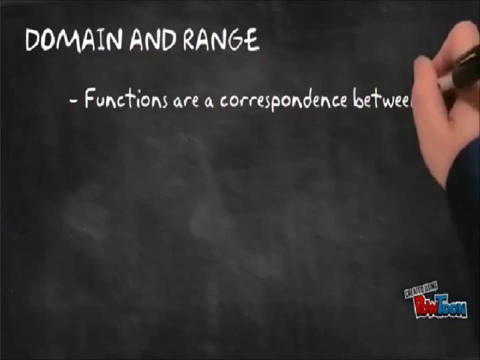 The standard form of quadratic function is: f of x is equal to ax squared plus bx plus c, and the vertex form is: f of x is equal to a times the quantity of x minus h squared plus k. Functions are correspondence between two sets called the domain and the range. 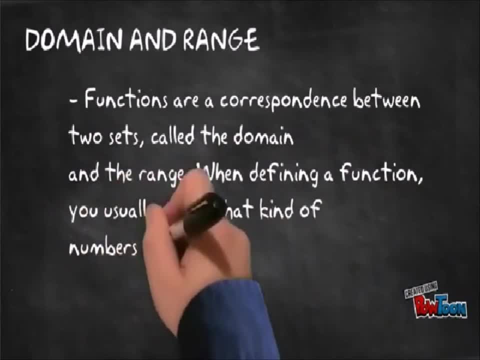 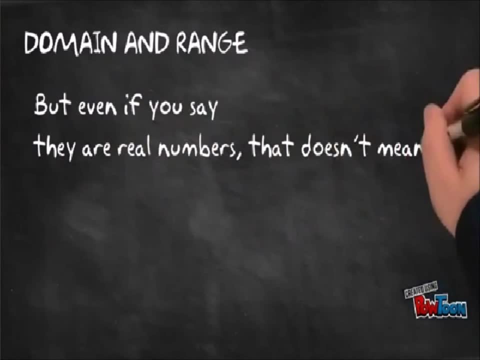 When defining a function, you usually state what kind of numbers the domain and range values can be. But even if you say they are wrong, you can still define them. If you say they are real numbers, that doesn't mean that all real numbers can be used for x. 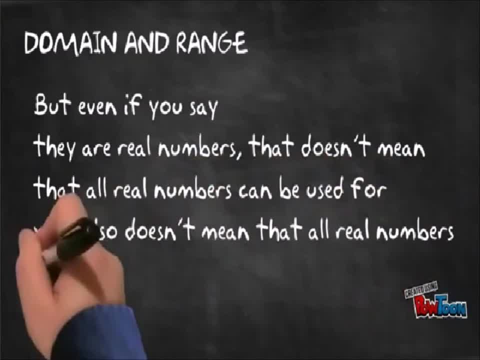 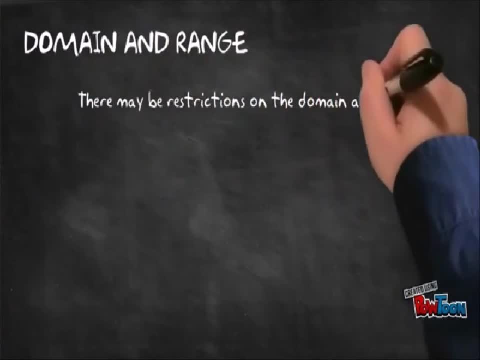 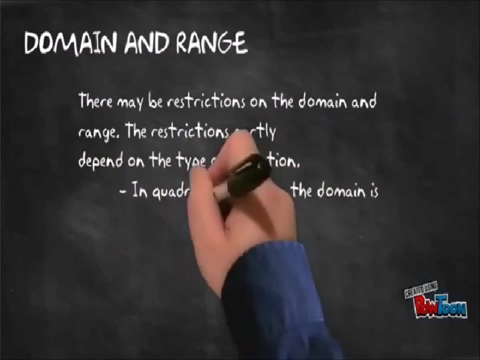 It also doesn't mean that all real numbers can be function values or f of x. There may be restrictions on the domain and range. The restrictions partly depend on the type of function. In quadratic function, the domain is always the set of all real numbers, or negative infinity up to positive infinity. 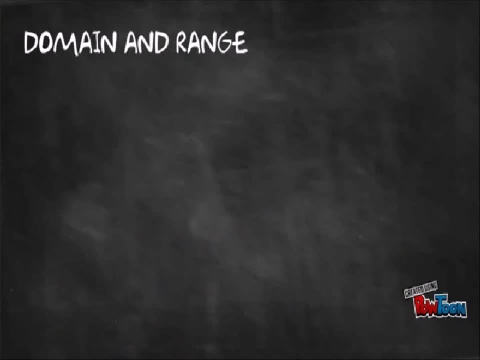 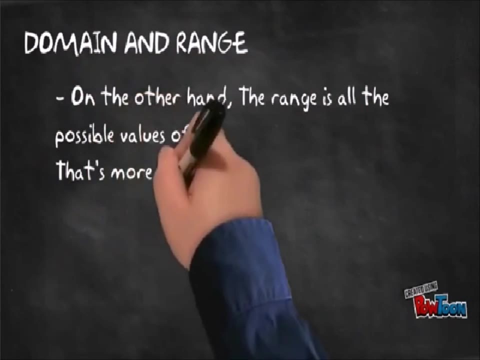 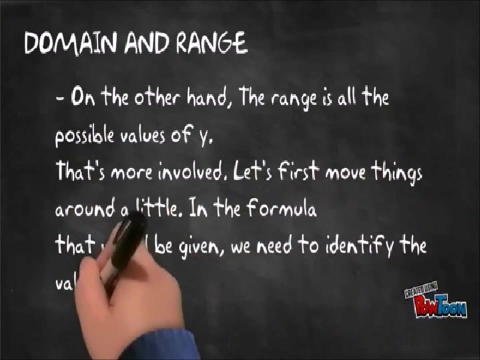 Which makes it pretty easy, as long as you remember that, On the other hand, the range is all the possible values of y. That's more involved. Let's first move things around a little. In the formula that would be given, you need to identify the value of a, b and c. 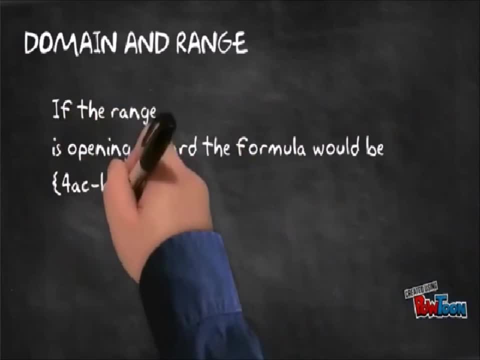 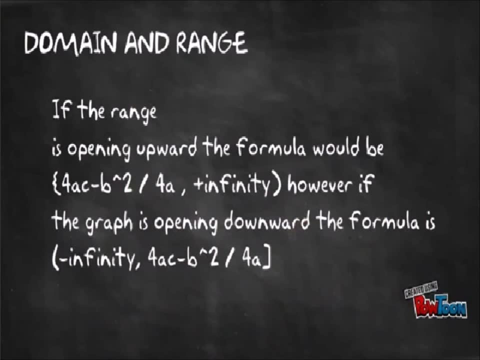 If the range is opening upward, the formula would be: quantity of 4ac minus b squared over 4a: comma positive infinity. However, if the graph is opening downward, the formula is negative infinity: comma 4ac minus b squared over 4a. 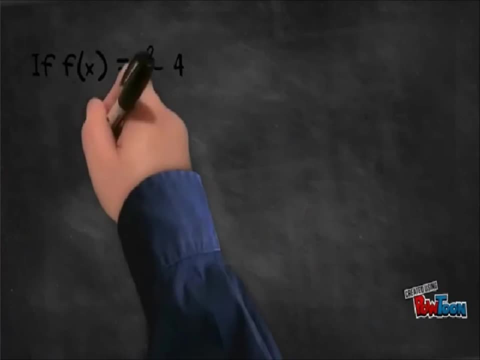 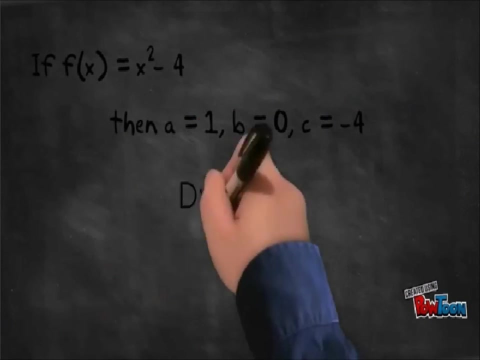 If f of x is equal to x squared minus 4, a is equal to 1, b is equal to 0, and c is equal to negative 4.. Since we already solved for the domain, we'll solve for the range. 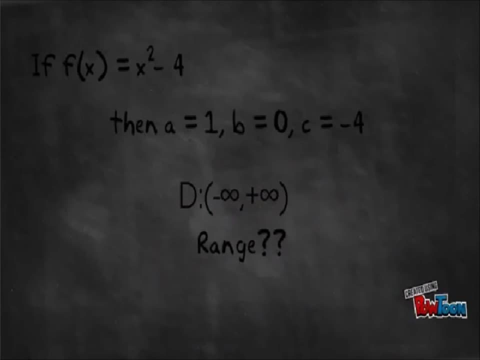 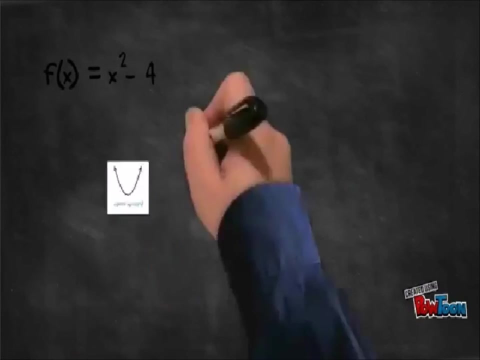 We need to find out if the graph is opening upward or downward. I'm going to tell you a little trick. Take notice of the x-value in the given function. If the x-value is positive, then it's opening upward. If it's negative, it's opening downward. 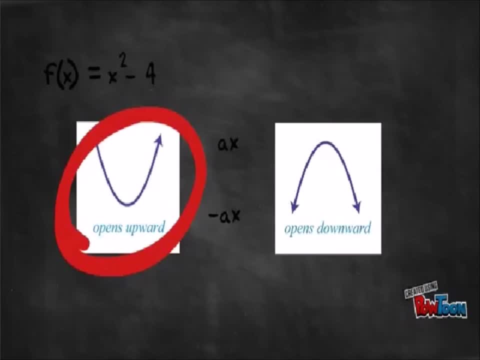 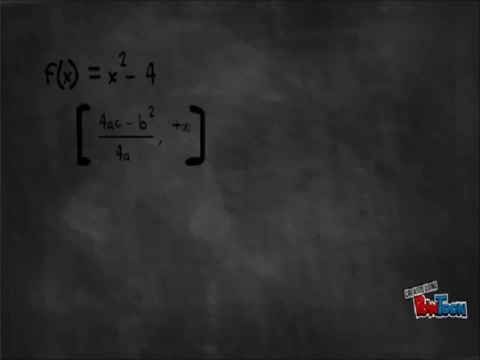 In our case, it is opening upward. Simple, isn't it? Since it's opening upward, we'll use the formula: 4ac minus b squared over 4a. comma positive infinity. Substitute the values of a, b and c to the formula. 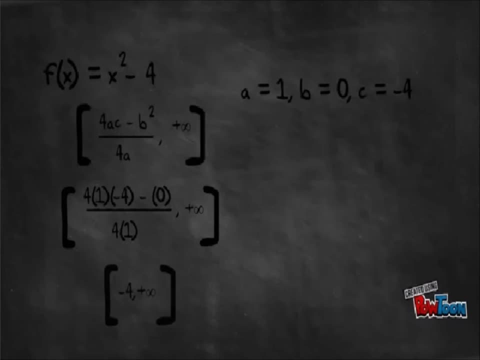 4 times 1 times negative, 4.. Minus 0, squared over 4 times 1, comma positive infinity is equal to negative 4, comma positive infinity. Now we'll go on to the next, which is drafting the function. 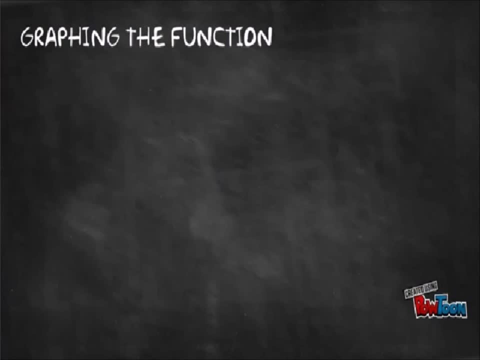 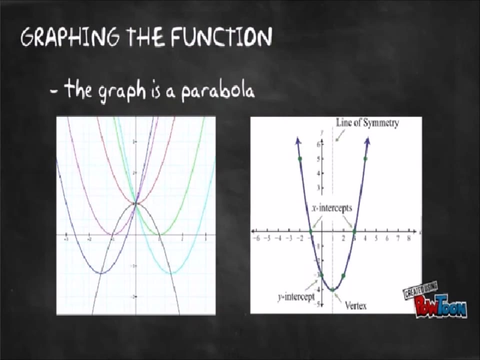 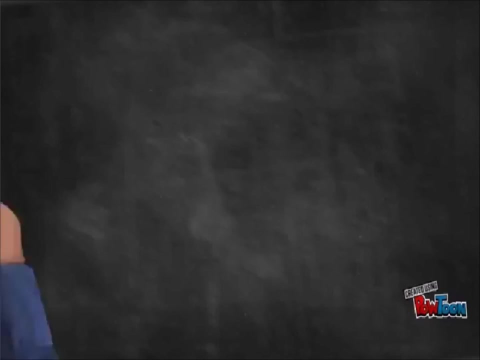 The graph of a quadratic function is a curve called a parabola. All parabolas are symmetric with respect to a line called the axis of symmetry. A parabola intersects its axis of symmetry at a point called the vertex. In graphing the function, we need to solve for its vertex first. 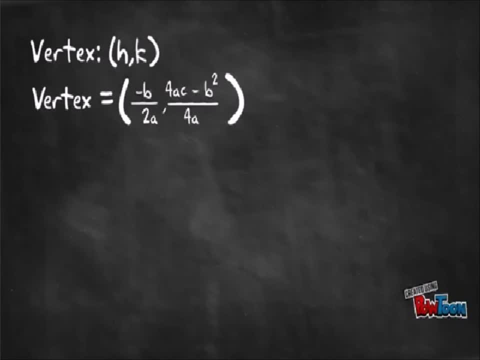 The formula in finding the vertex is negative: b over 2a, comma 4ac minus b squared over 4a. Now look at the formula. Can you see something familiar? Yes, because the formula for solving the y in our vertex is one of the formula we used earlier. 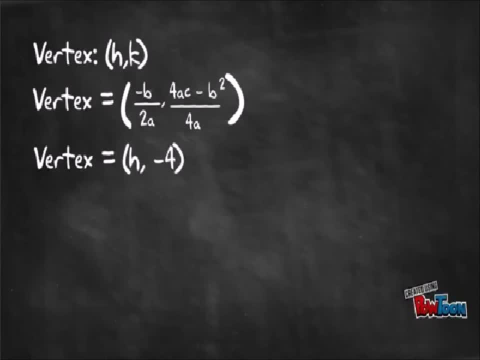 Because we already solved for the y, we'll solve for x, Just like what we did before. substitute the value of a, b and c And we'll get the formula 0,. comma negative 4 is the vertex of the function. 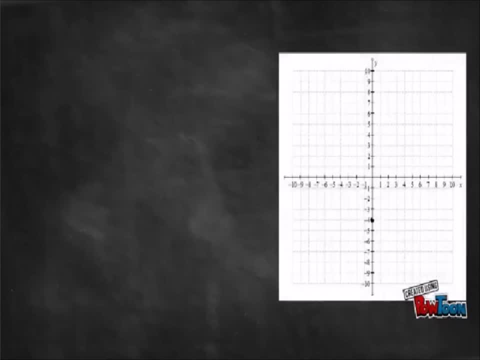 But we can't stop there. The next thing we need to do after you've plot the vertex, is to find the x-intercepts. To do that, we need to equate the given functions to 0.. If f is equal to x squared minus 4,. 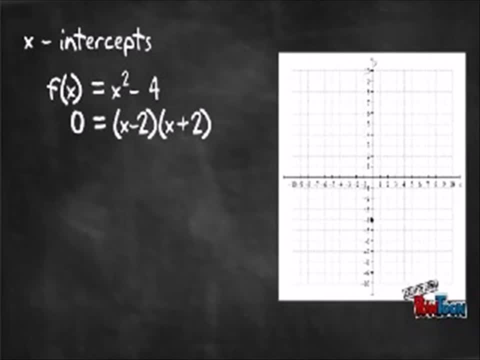 replace f with 0, and factor out x squared minus 4.. 0 is equal to the quantity of x plus 2 times the quantity of x minus 2.. x is equal to 2, and x is equal to negative 2.. 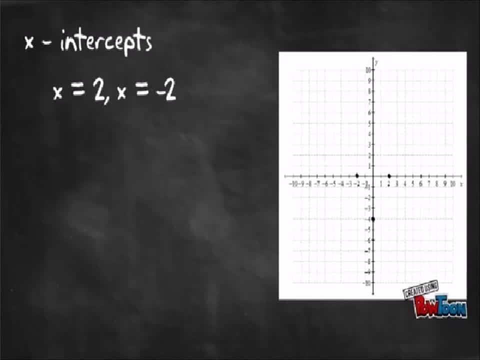 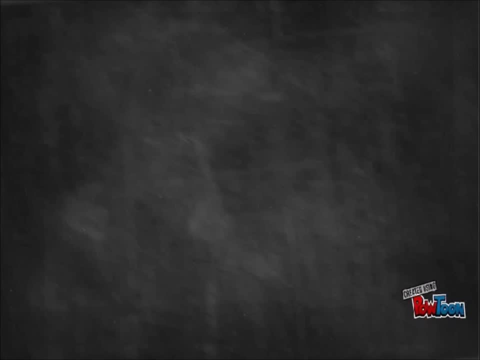 After finding the x-intercepts, plot it on a graph, Connect the three dots we solved for, and then we're done. Don't you know that quadratic functions can be applied in real life, Just like in your favorite game of basketball? quadratic functions can be applied. 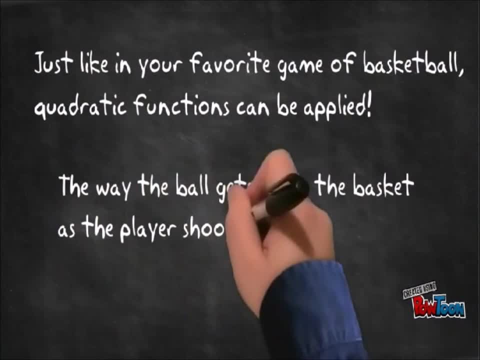 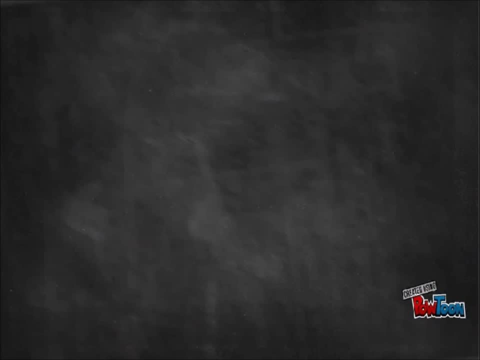 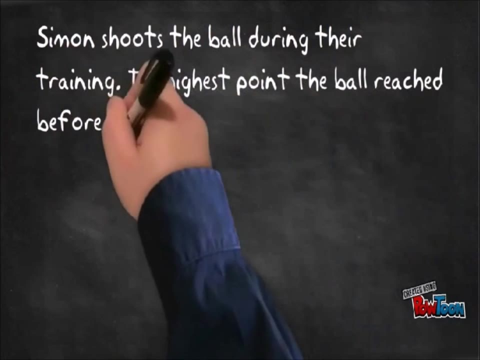 The way the ball gets inside the basket as the player shoots. it is parabolic in nature. Simon shoots the ball during their training. The highest point the ball reached before it went inside the basket is 10 meters in height and 5 meters in distance. 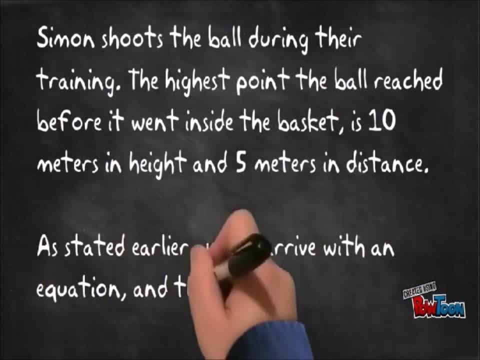 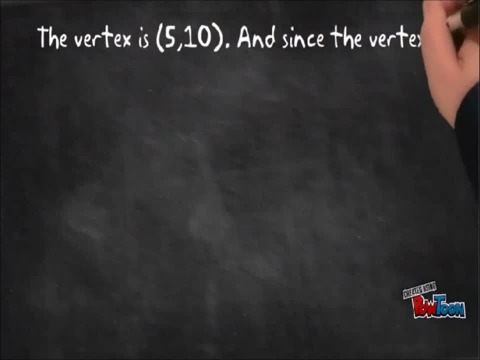 As stated earlier, we can arrive with an equation, and that's what we're going to do. The vertex is 5 comma 10, and since the vertex is given, we can use the vertex form of the function. f is equal to the negative quantity of x minus 5, squared plus 10.. 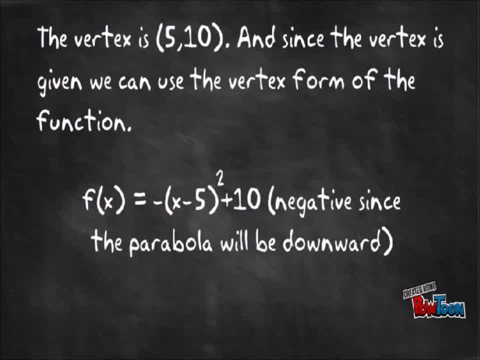 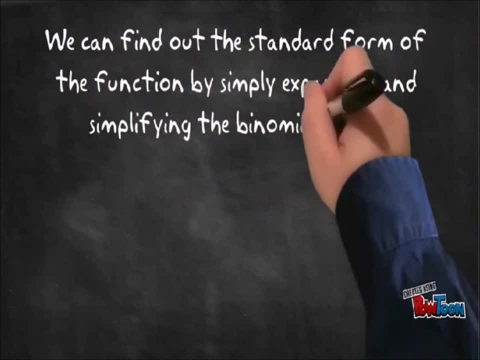 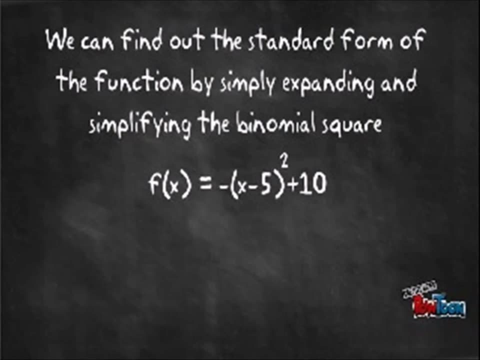 Negative. since the parabola will be down, We can find out the standard form of the function by simply expanding and simplifying the binomial square. f is equal to negative quantity of x minus 5. squared plus 10, is equal to. f is equal to negative quantity of x minus 10x plus 25 plus 10.. 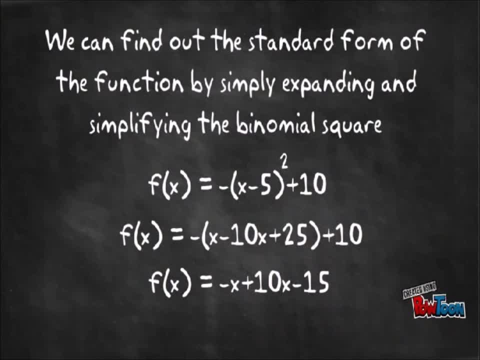 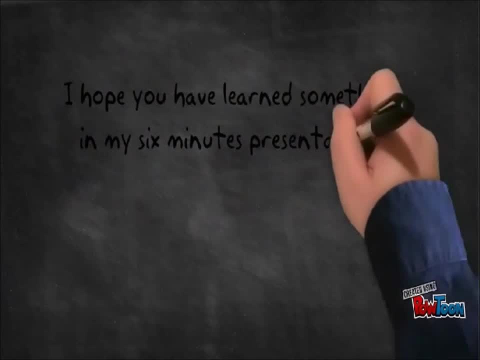 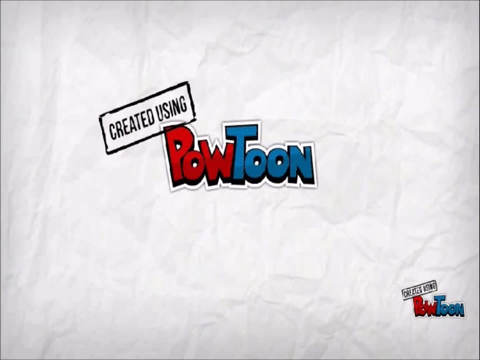 f is equal to negative x plus 10x minus 15.. I hope you have learned something in my 6 minutes presentation. Thank you for watching. Created using Powtoon.